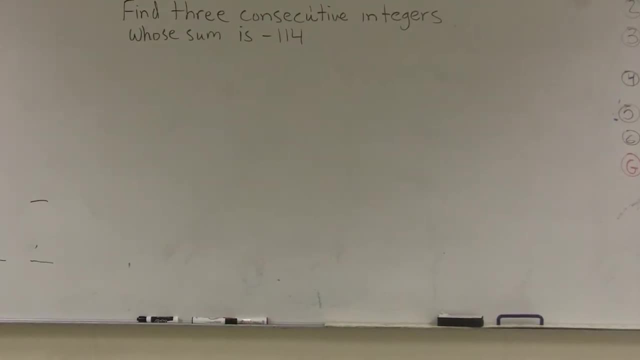 All right, What I'd like to do is show you guys how to find three consecutive integers whose sum is negative: 114.. So the first thing we need to do is we need to understand what consecutive are, And if I was going to write consecutive numbers, let's say this is 1, 2, 3, 4, 5, 6,. 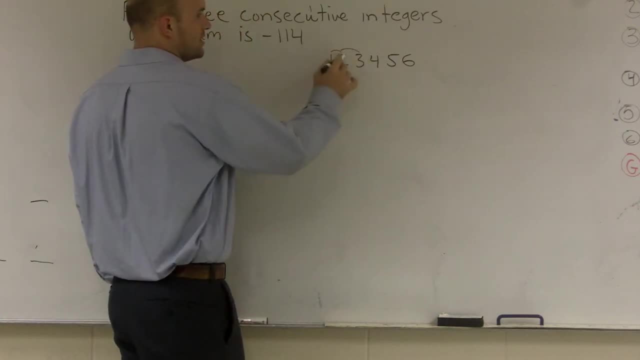 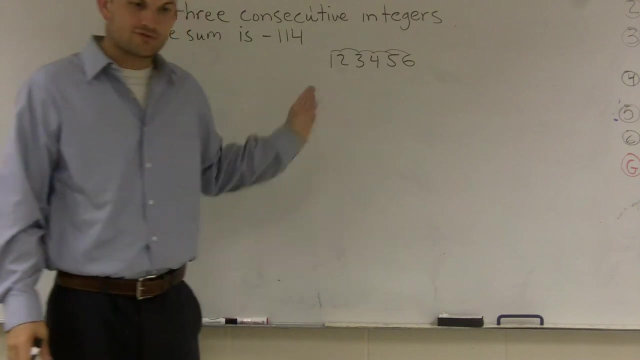 consecutive numbers are numbers right next to each other. So 1,, 2,, 3,, 4,, 5, 6, these are all consecutive numbers. They consecutively go to the next number. Now the next thing is find three consecutive. I don't think I wrote this down right. 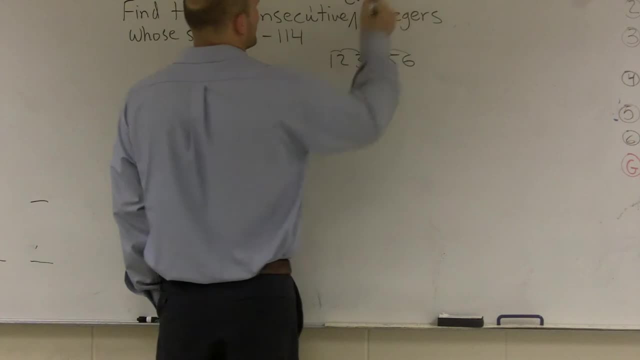 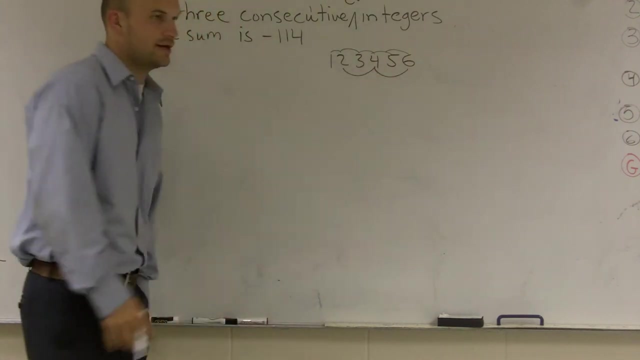 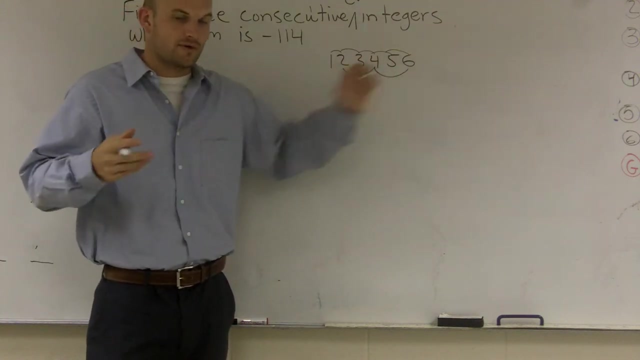 Yes, I didn't. Let's call it even numbers, So let's do three consecutive even numbers. So therefore, I need to do 2,, 4, and 6.. All right, See how these are consecutive even numbers. They're even numbers right next to each other. as far as the next even number would be consecutive, 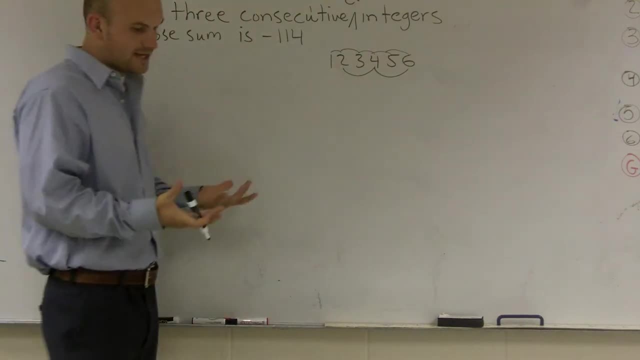 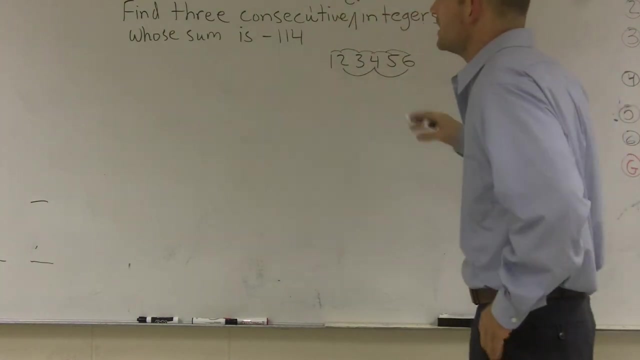 So what the problem is asking is: I need to find three numbers. Now, when we're doing a word problem, we need to make sure we understand first what the question is asking. This says we need to find three consecutive even numbers. That means my answer: I'm going to have to have three even numbers. 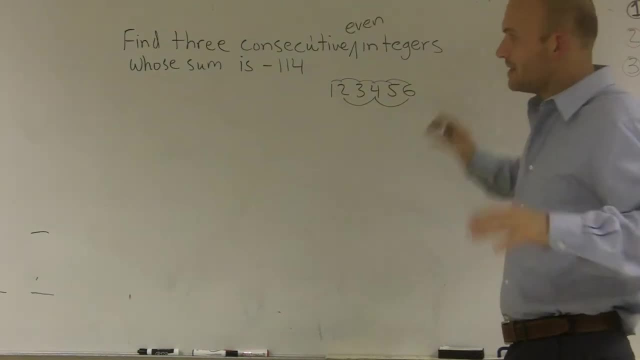 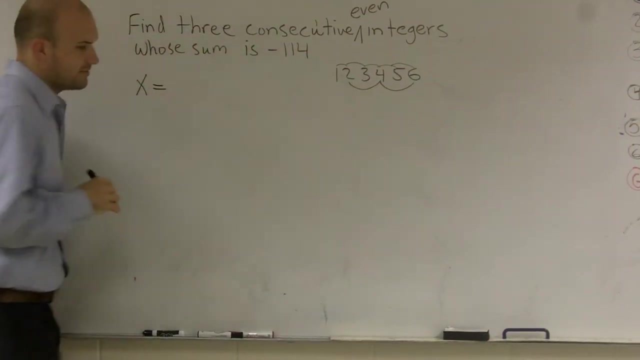 The next thing is we're trying to find a word problem. we're going to have to distinguish what we want to solve for. So I'm going to say I'm going to make it x and I'm going to say: what does x want of equal? 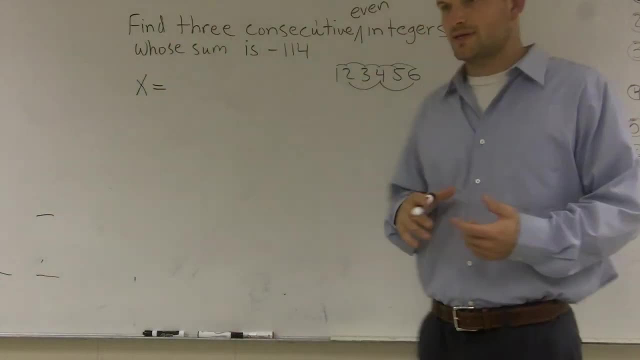 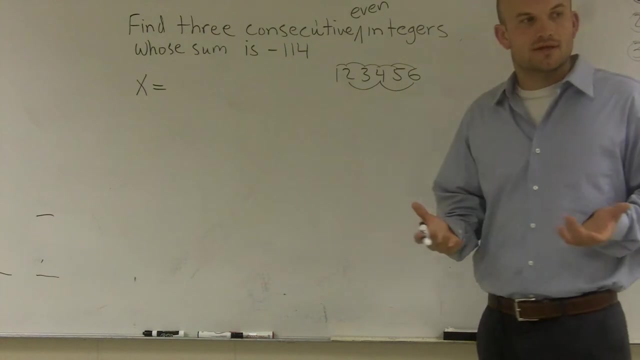 Well, I can't have x equal to x. I can't have x equal all three of those numbers, because if I just said x plus y plus z equals negative 114, how do you solve for one of those variables? So what we want to do is we want to create one variable. 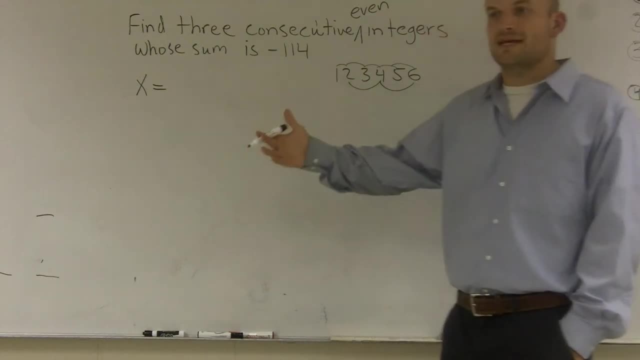 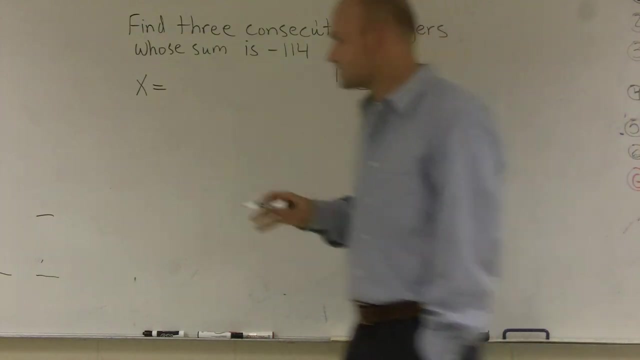 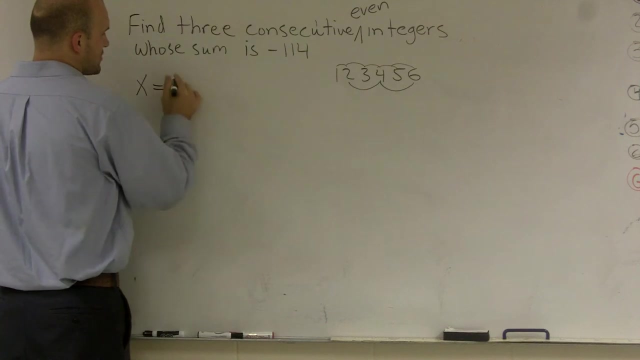 have that represent something and then relate the rest of our unknowns to that one variable. So if that's kind of not making some sense, let me see if I can explain this. Let me see if I can show you. Let's have x represent. x equals the first even number. 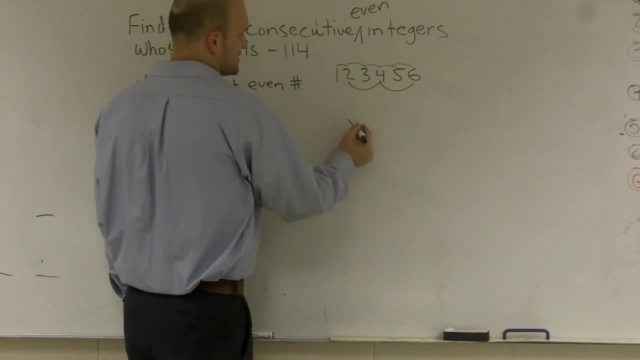 So let's say x equals the first even number. So let's just say it's x. Well, if you guys don't understand what consecutive numbers are to go from my first number, let's say my first number here is 2.. 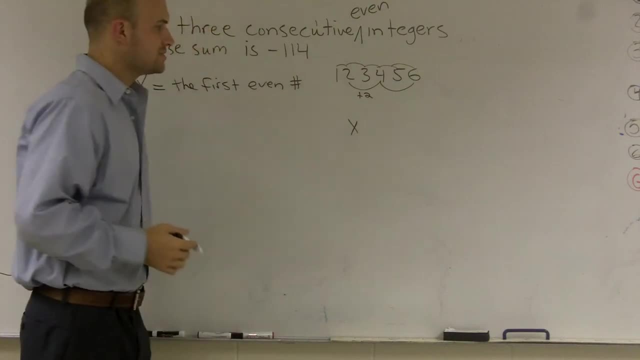 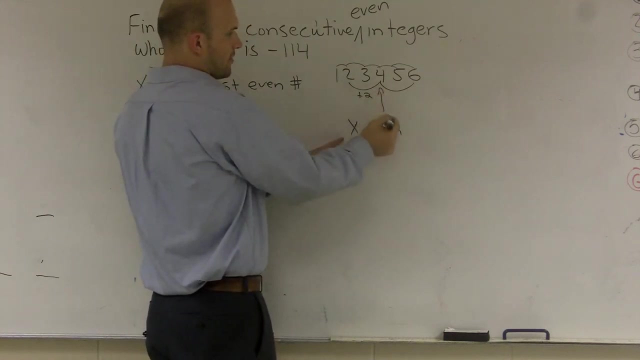 To get to my next number, I have 2 plus 2.. So if my first number is x, my next number would be x plus 2.. That would be 4.. And then I have to add 2 again to get to 6.. 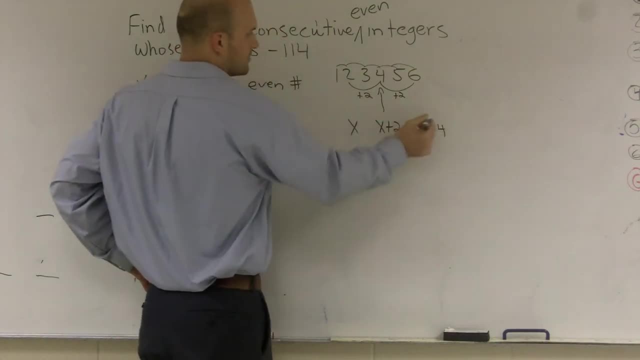 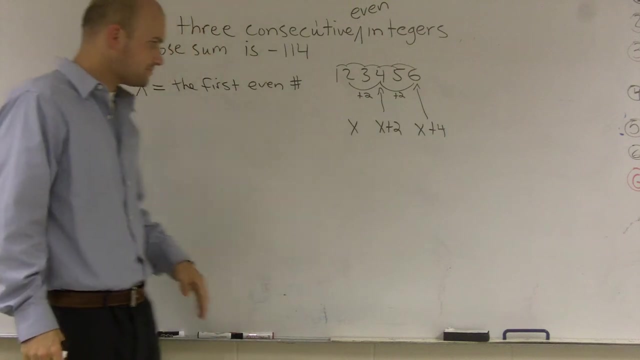 So then my third number would be x plus 4.. Now in here, in this example, my first number was 2.. But I don't know what my number is. I don't know what my first number is. That's why we gave it x. 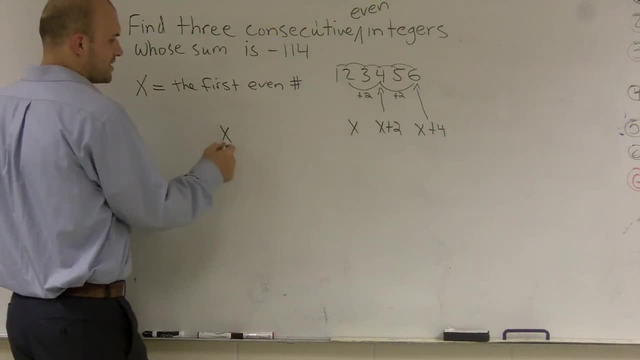 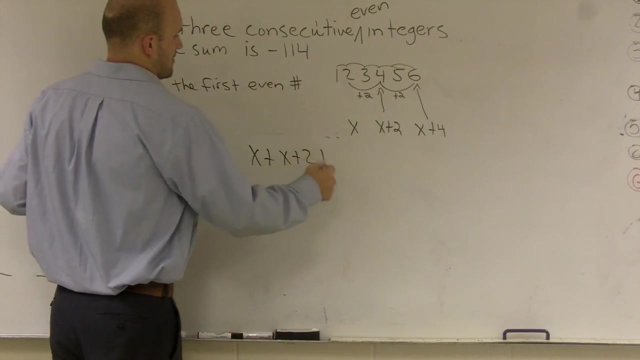 Now it says the sum of them. So sum is going to tell me addition. So I can write x plus x plus 2 plus x plus 2.. Plus 4 equals- now I ran out of room- equals negative 114.. 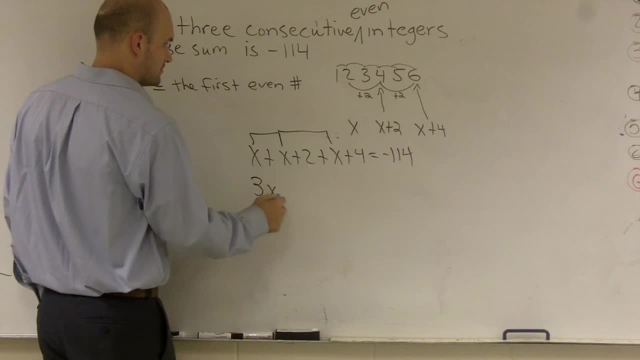 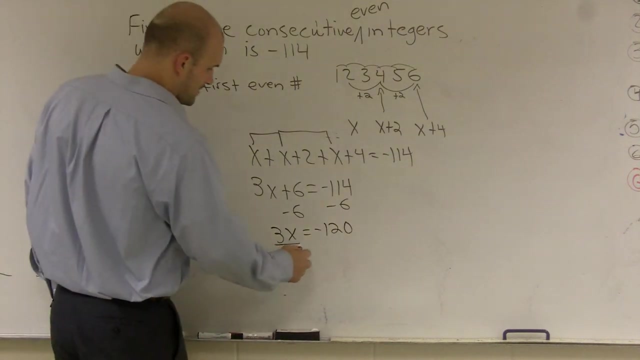 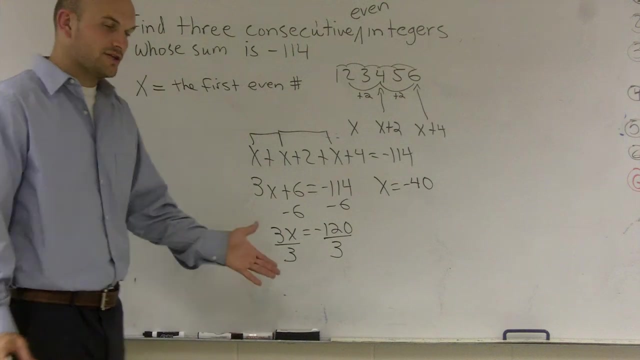 I can combine my like terms. subtract 6,, so x equals negative 120.. Divide by 3. And what I get is x equals a negative 40.. Now the next thing we need to do is that was sort of x equals. 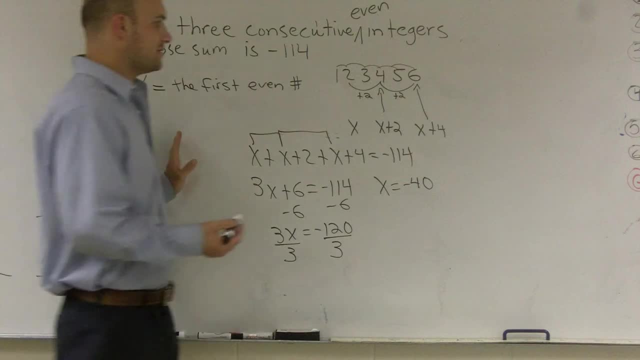 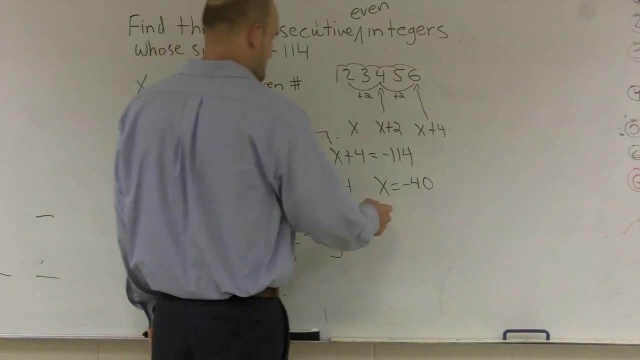 So, therefore, my first number is negative 40. However, remember, if x equals negative 40, then the next number is going to be negative 40 plus 2, which will give me, so I can say, my first number. let's just write it over here. 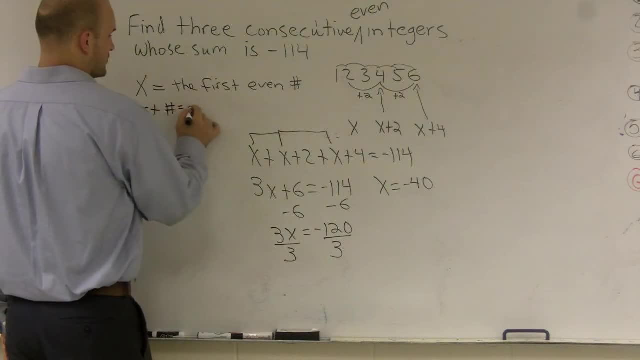 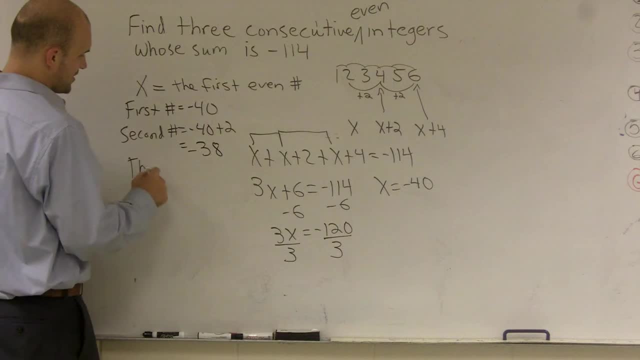 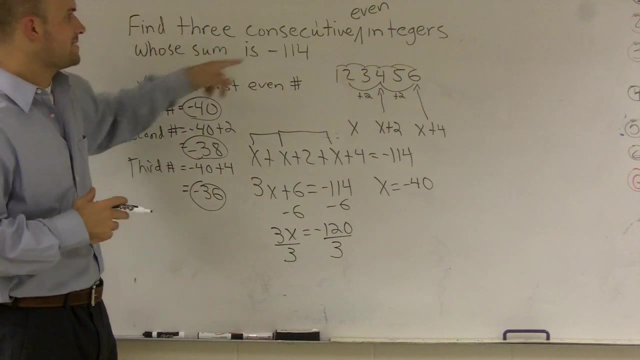 which is equal to a negative 38.. And my third number is negative 40 plus 4,, which is equal to a negative 36.. Therefore, the three numbers consecutive, even numbers that add up to negative 114,. there are negative 40, negative 38, and negative 36..